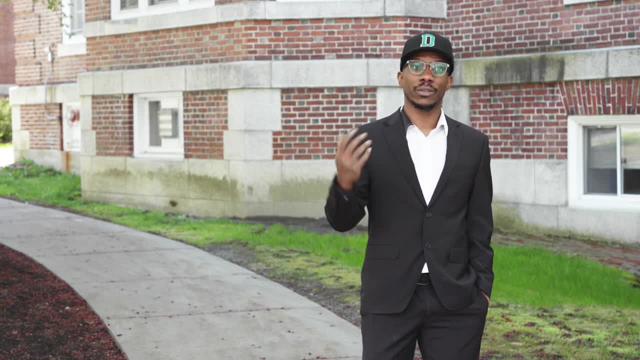 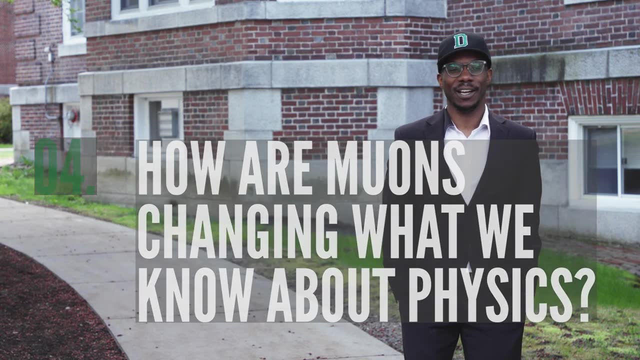 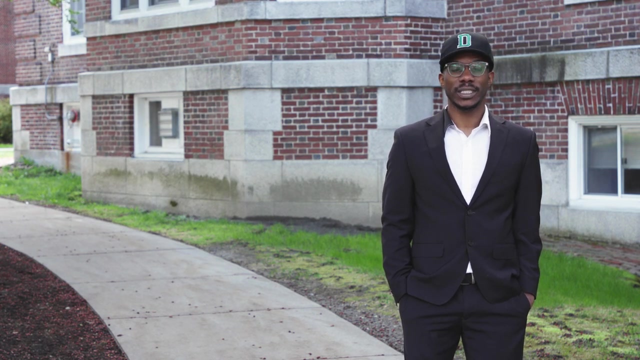 first discovered And again, as I mentioned, they can be generated inside of lab conditions now. So this is a really interesting question. The announcement came out the day before we were discussing the electron spin g factor, So the experiment that was confirmed recently was the. 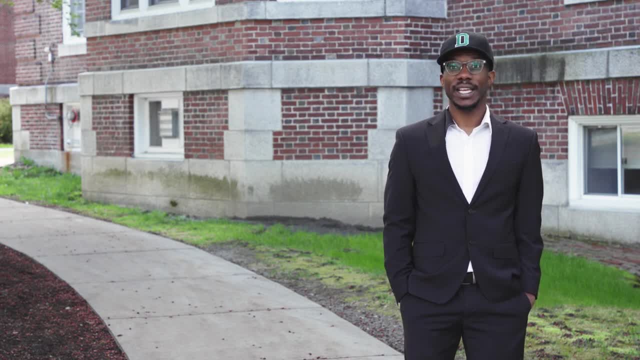 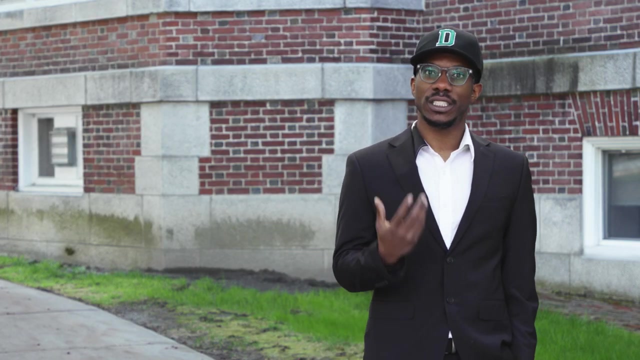 muon g2 experiment from Fermilab And they discovered a discrepancy from what was the theoretical calculation. The theoretical calculations for the same g factor for the electron was the subject of the 1965 Nobel Prize And in that they found that the g factor of the electron was slightly off And this g factor of the electron 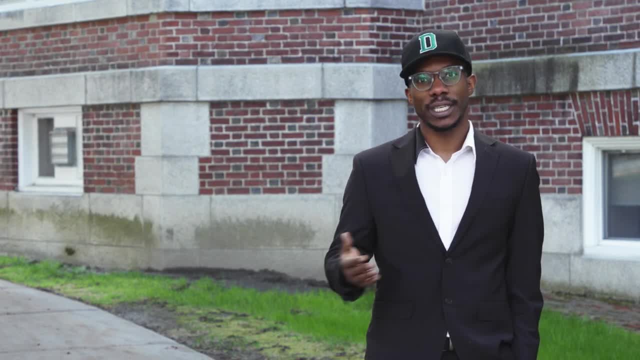 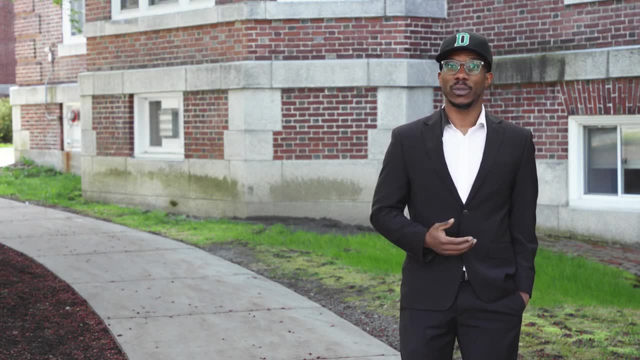 this anomalous magnetic moment was calculated using quantum electrodynamics, using very sophisticated mathematical techniques, And what people have discovered was that the muon corrections are not consistent with what they expected to find, And that's what we're going to talk about today. 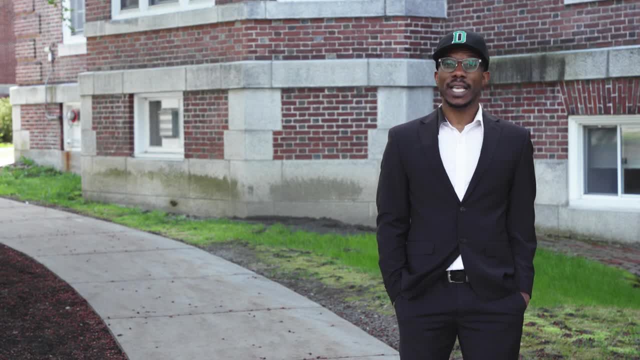 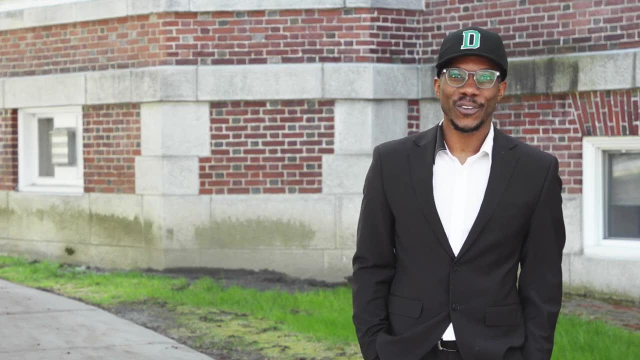 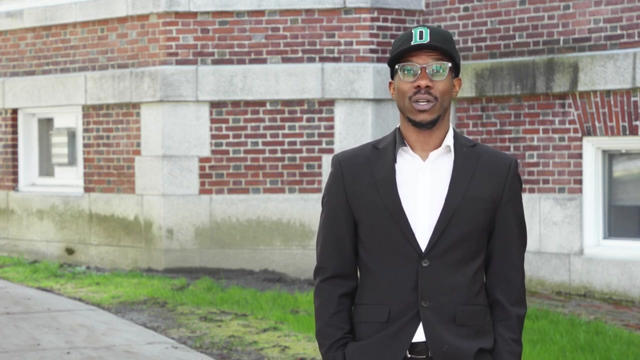 From the standard model of physics, So this is actually interesting because this was already known. This is just a confirmation of the discrepancy based on recent data. In our physics 40 class, the quantum physics of matter, we discussed the electron g factor the day before this experiment. 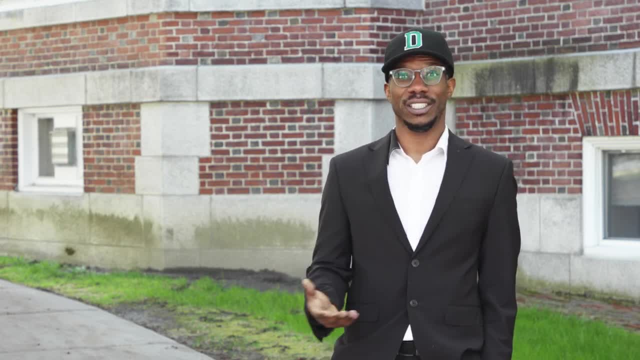 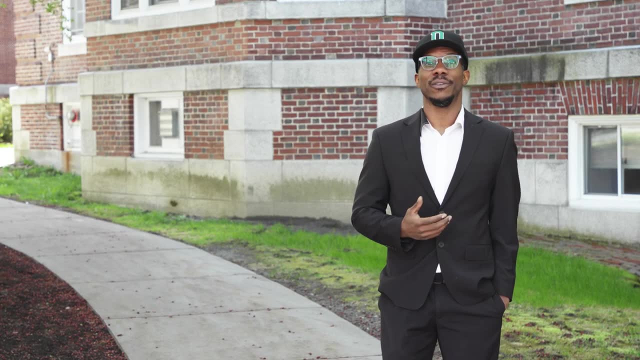 was announced. It was very exciting to be able to take our discussion of the g factor inside of class, of the electron g factor and its anomalous magnetic moment, to understand the anomaly of the muon magnetic moment, Which is also calculated using quantum electrodynamics, as well as other corrections. 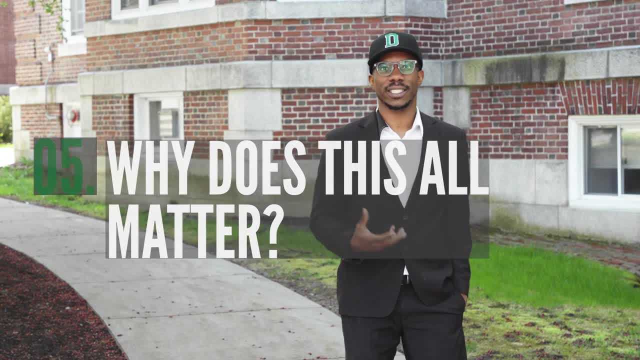 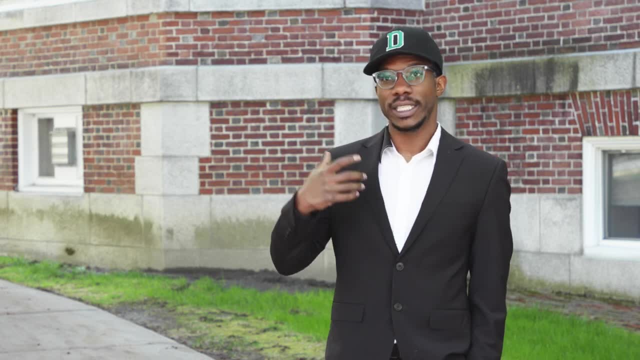 So this is really interesting because this gives us a really interesting way to test fundamental physics. So when we think of physics, atoms in the gas around us, electrons, dictate a lot of the atomic structure around us. We understand a lot about the atoms. We talk about chemistry and 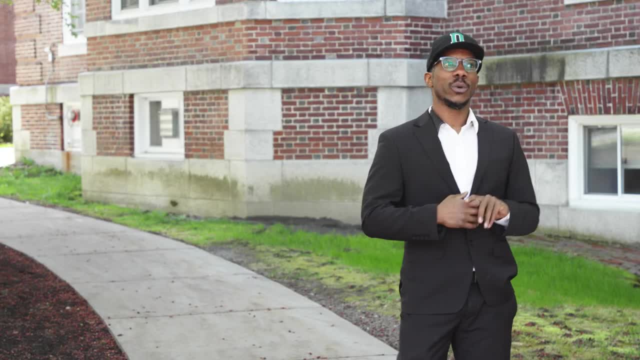 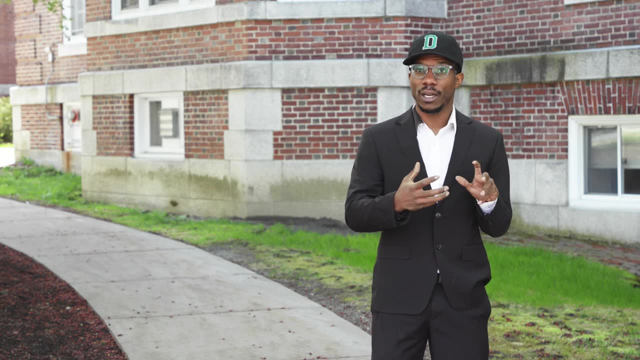 biology in terms of the atoms that are there. If we want to understand the fundamental particles, we end up with a whole new table of particles that are going to dictate the binding of nuclear matter, And understanding this binding of nuclear matter will hopefully allow us to invent new technologies, understand how to use these things for better science, As I mentioned.